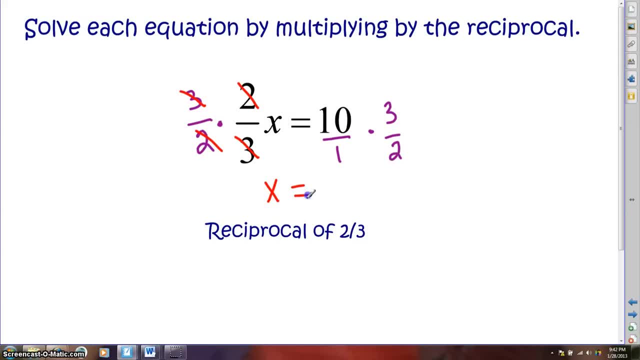 and that will leave us just the x, which is what we want. So we're trying to isolate that variable. we can reduce the 10 and the 2 and we get the whole number 15.. Let's try another. This time we're going to multiply by the reciprocal of 3 fourths. 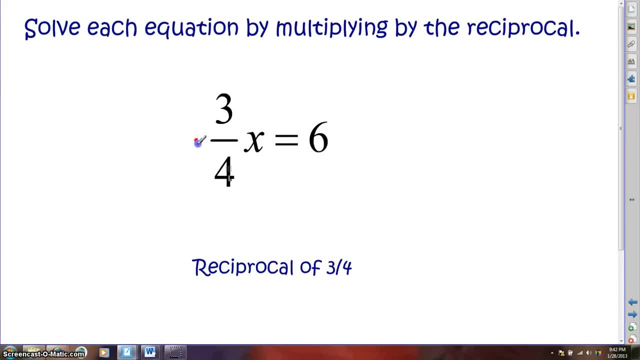 So the reciprocal of 3 fourths is 4 thirds. So over here on the left we're going to multiply by 4 thirds, which means we have to come over here on the right and multiply it by 4 thirds as well. So on this side, our fractions. 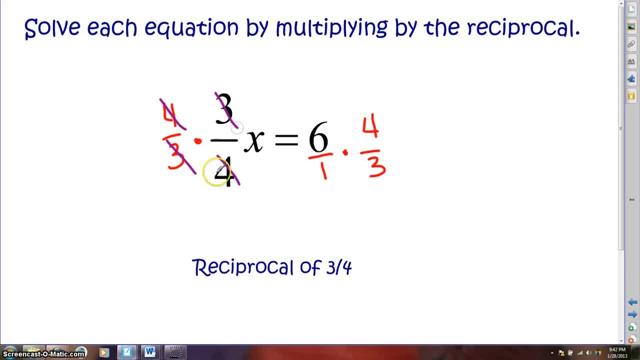 cancel out. The 4's cancel out, The 3's cancel out. So we have just the x left and over. here we can reduce the 6 and the 3.. Leave me a 1 and a 2. So 2 times 4 would. 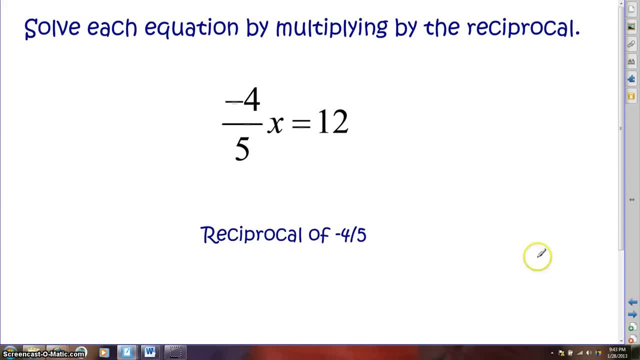 make 8.. Let's try just a couple more. So we have negative. 4 fifths x equals 12.. So we're going to multiply by the reciprocal. So we flip that upside down and we multiply by the reciprocal. So we flip that upside down and we multiply by the. 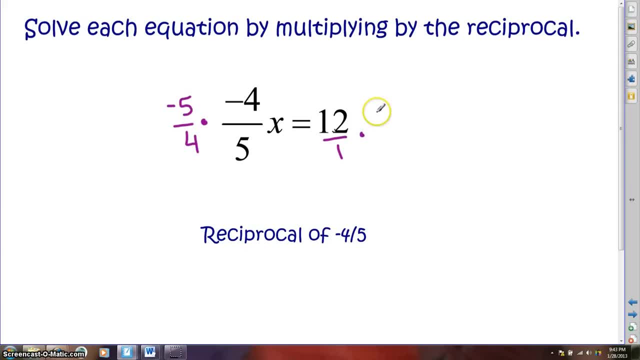 negative 5 fourths, And that means we multiply the right-hand side by negative 5 fourths as well. Negative 5 and the 5 reduce to negative 4 and the 4. And since those were both negatives, that makes us have a positive, And over here we can. 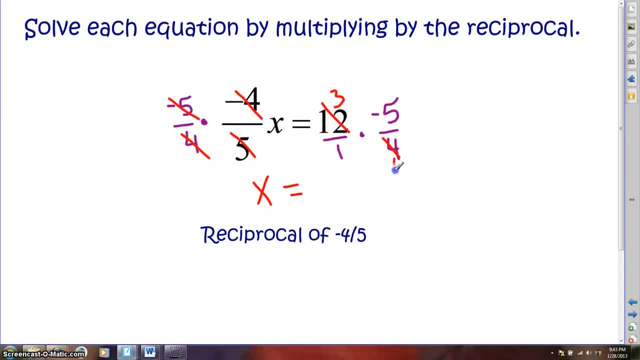 reduce the 4 and the 12.. 12 becomes a 3. The 4 becomes a 1. And a positive 3 times a negative. 5 makes a negative 15.. Let's try one last question: Reciprocal of 3 fifths. Flip that upside down, Which means: 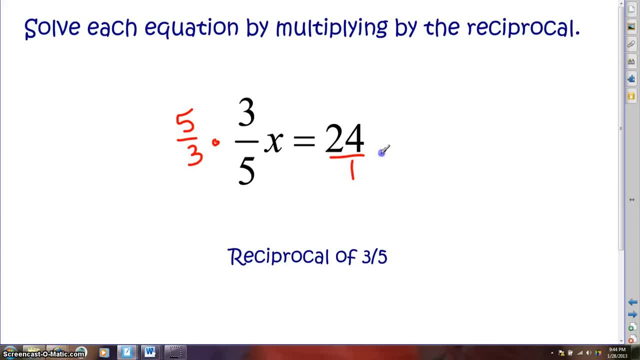 we are multiplying by 5 thirds, and if we multiply this side by 5 thirds as well, The 5's cancel out, The 3's cancel out. So on the left we just have an x, and over here on the right those will cancel, We get a 8.. 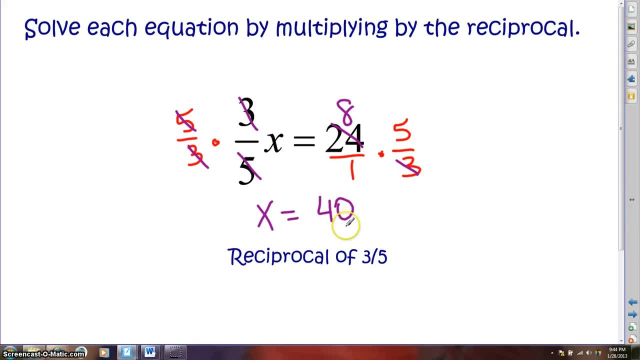 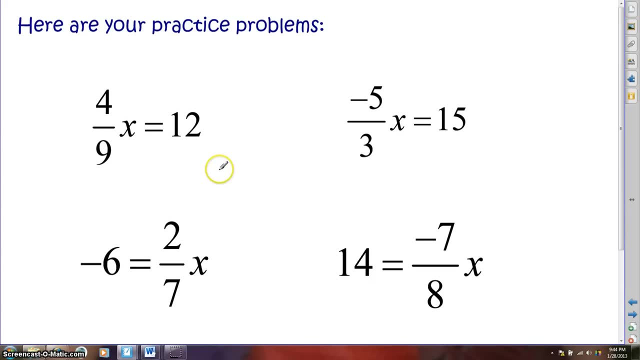 8 times 5 makes 40.. All right, now it's your turn to try. Here are your 4.. So in the boxes at the bottom of your sheet, fill in with these questions: 4 9ths x equals 12..